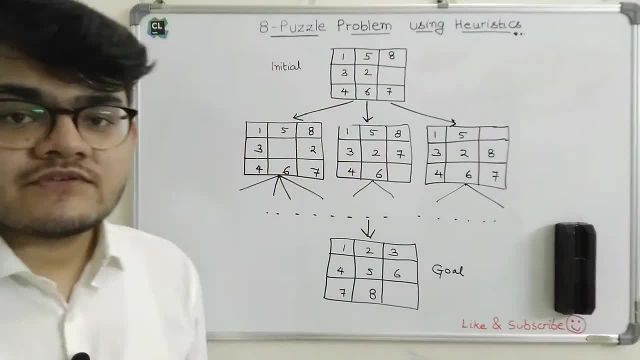 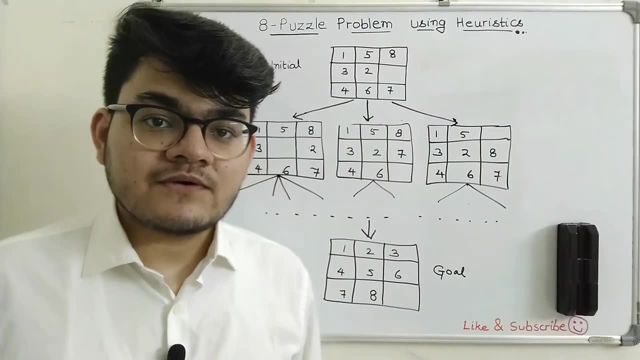 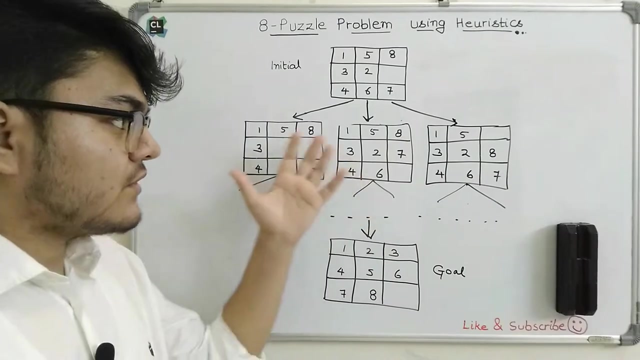 Right. So I have picked a very simple game which is an 8 puzzle game or an 8 puzzle problem, and we are going to see how we can use heuristics or the heuristic function to make sure that the AI agent does not traverse all the branches inside of the problem. 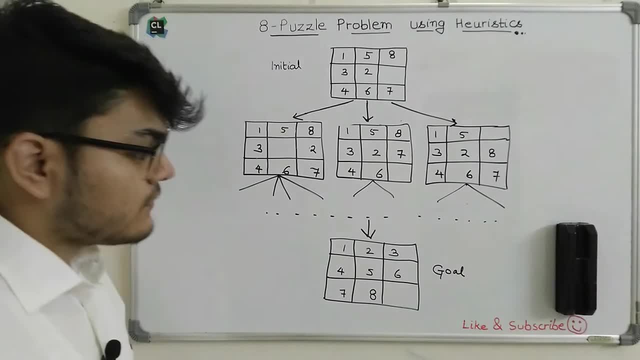 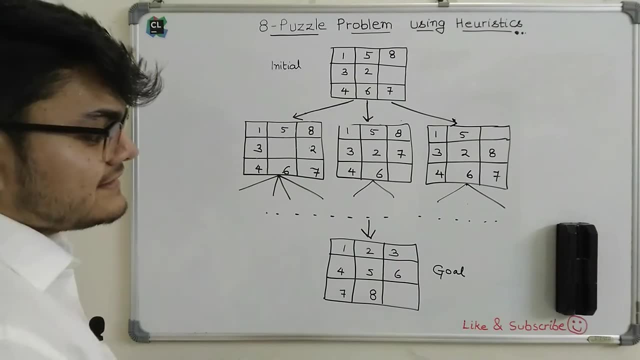 Right, So let's start with this now. So, first of all, the problem, or the game, is like this: Initially, let's say, we have a state, something like this: The final state That is required, which is the goal state. 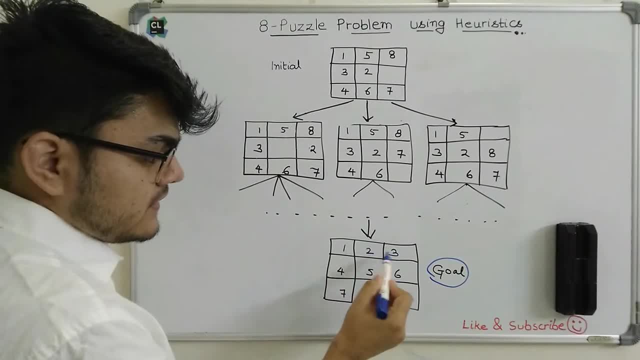 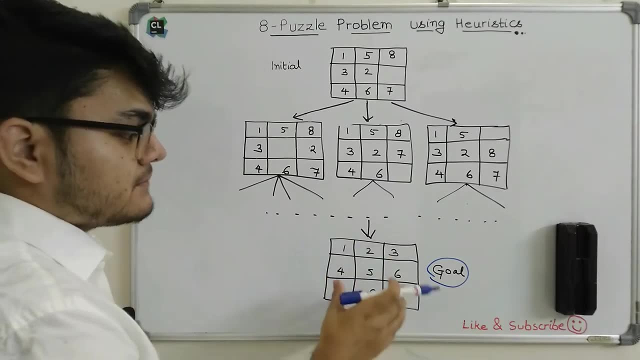 Here you can see this. It is 1,, 2,, 3,, 4,, 5,, 6,, 7,, 8 and a blank space. It is known as the 8 puzzle problem or 8 puzzle game. 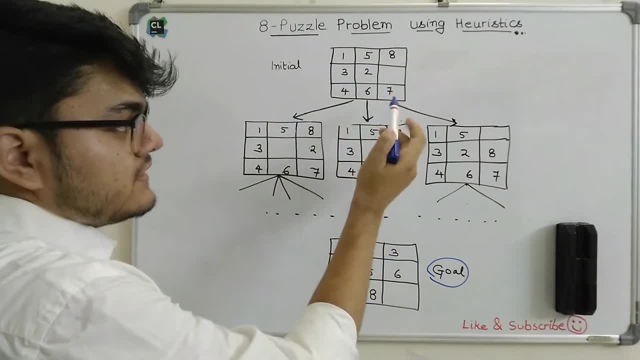 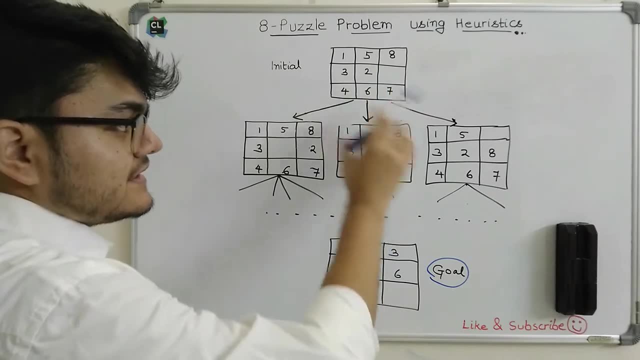 So what we need to do is we will have to move. We are actually free to move these elements here, So I can move 7 here or I can move 2 here, And using these movements, we will have to get this type of configuration. 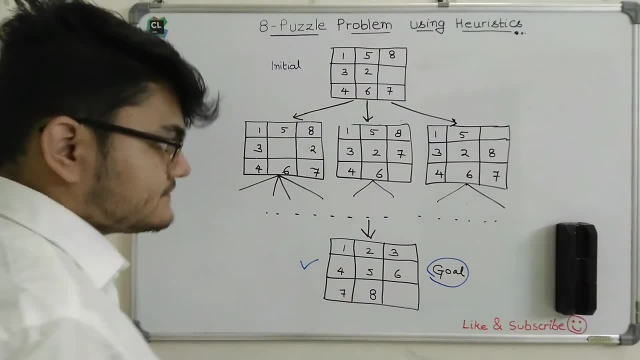 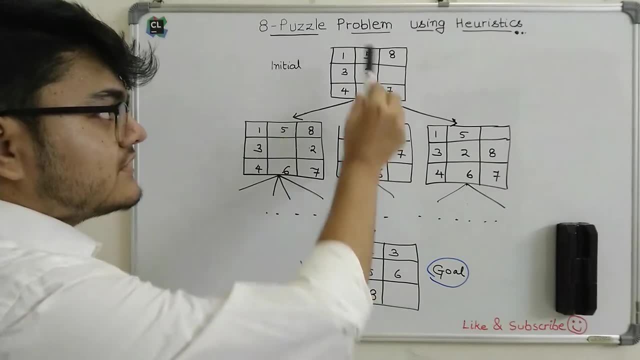 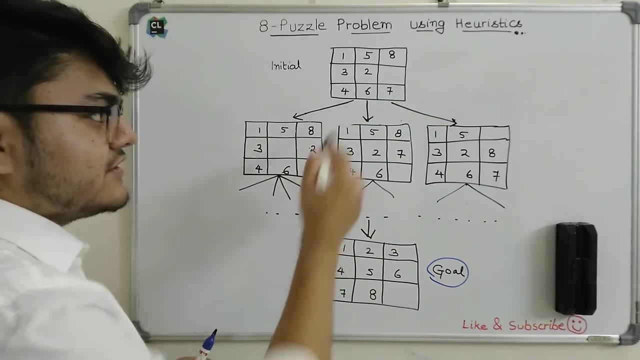 This is basically what this game is all about, Right, All right. So let's start with the state space representation of this problem, which is essentially used by the AI agent, Right, Right? So let's say the AI agent is at this place initially. 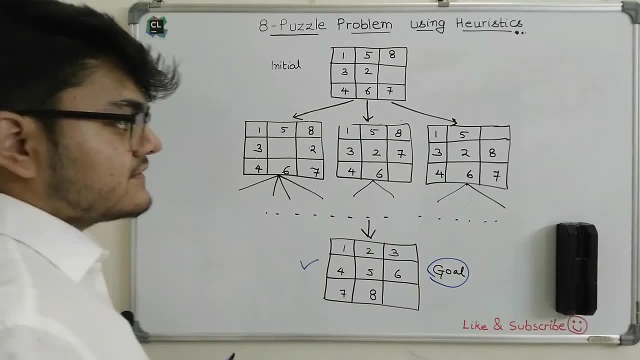 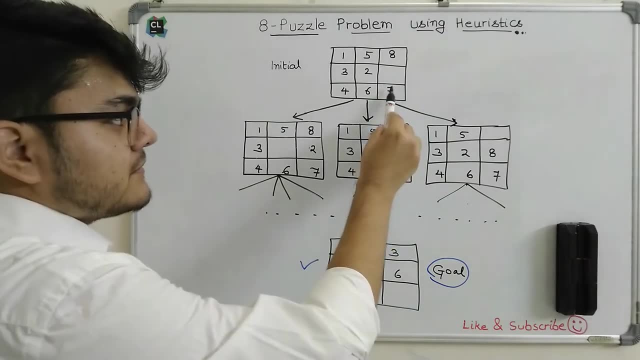 Now, from here, we can have three different states. What are these states? You can see if I can move 7 up here- Right. So if I move 7 up here, Right, I will get this type of state. You can see now. 7 is up. 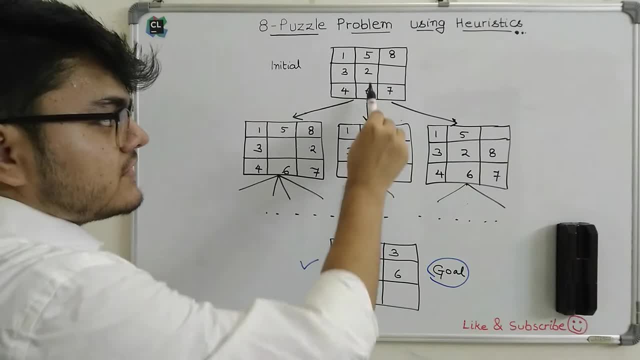 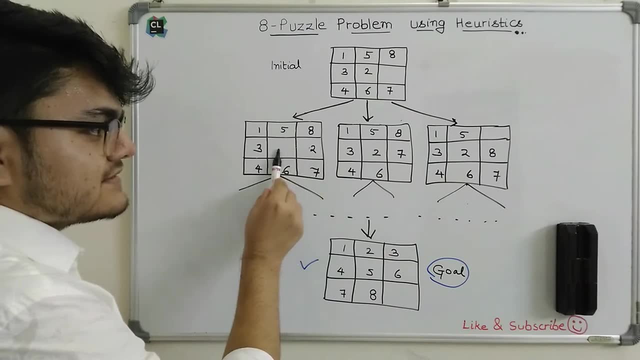 So the blank space is now down. Second configuration is: 2 can move here. Right, So you can see this in this configuration. 2 has been moved here, So the space is here. In the third configuration: I can move 8 here. 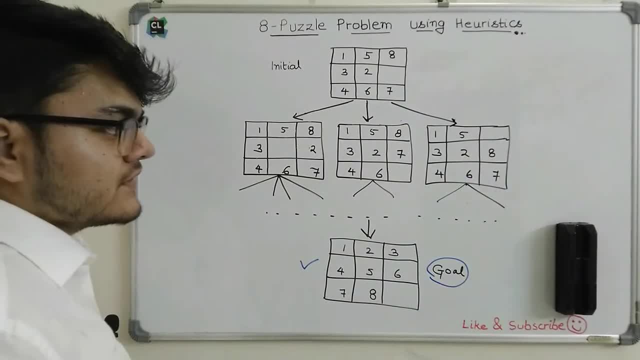 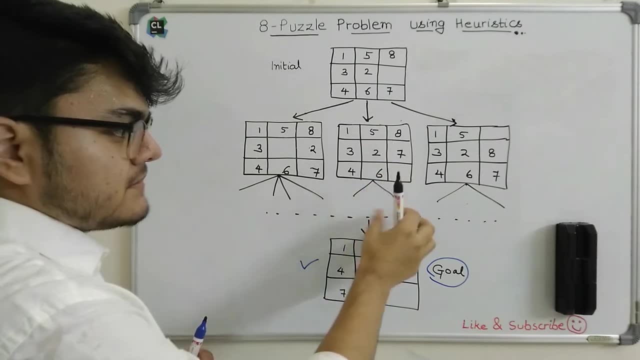 So 8 is now here and blank space is upwards. So you can see that these are the three possible combinations that I can get. I will keep breaking this into Branches Right. So at this step you can see we have this space. 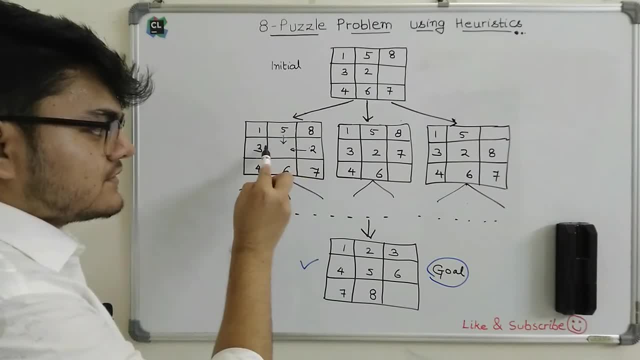 So 5 can move here or 2 can move here, 3 can move here and 6 can move here. So there can be four different possible branches here. You can see: 7 can move here, 6 can move here, So there are two possible branches. 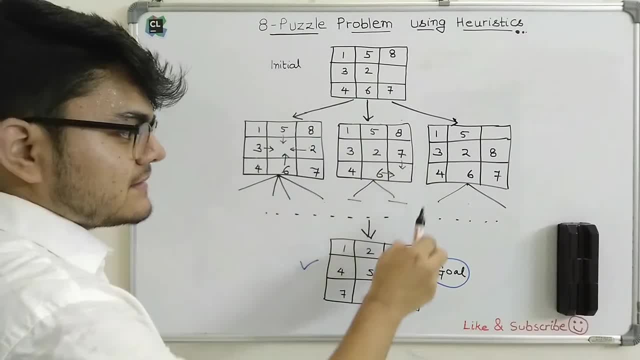 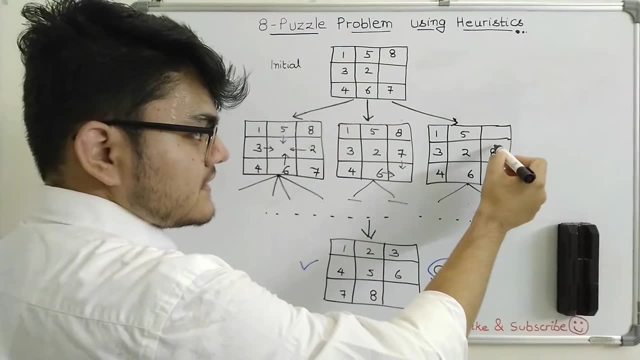 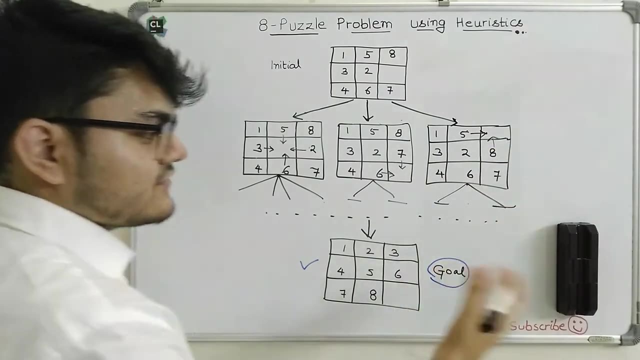 We can draw these states, as we have done in this step. We can do this recursively and then, finally, we will be able to reach the goal Right Now. here you can see, 8 can move here and 5 can move here, So we have basically two more different combinations or states. 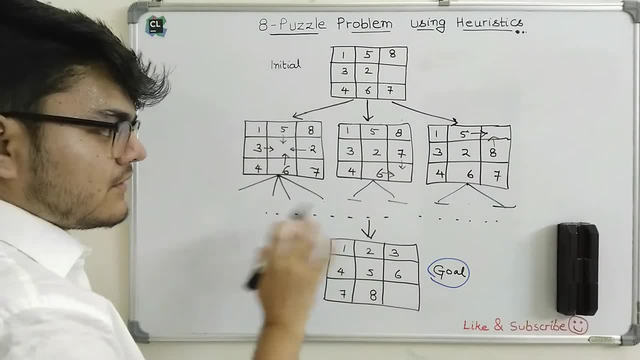 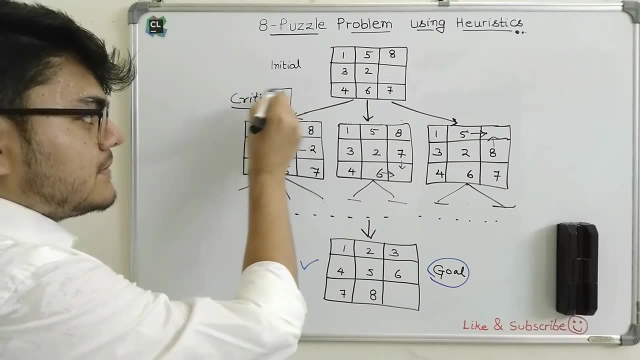 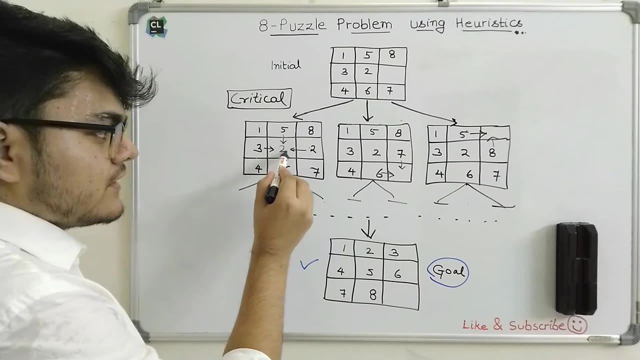 Right Now one important optimization, or I should say a critical optimization in this problem, that we are going to make an assumption that you can see that if I try to move to here, Right, Let's say I move to here, So this will become the blank space. 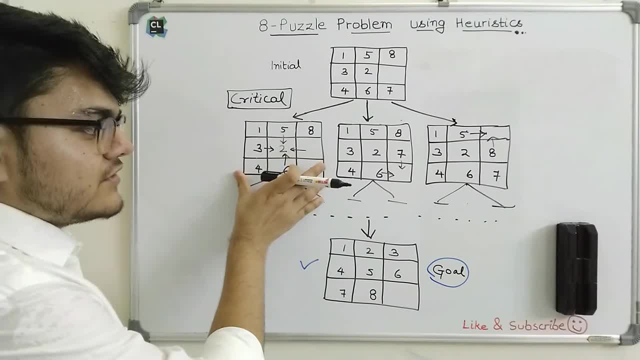 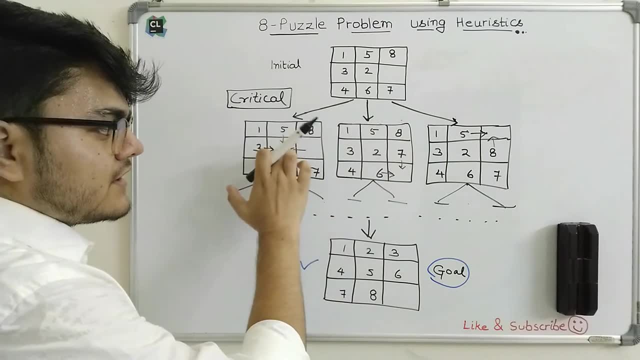 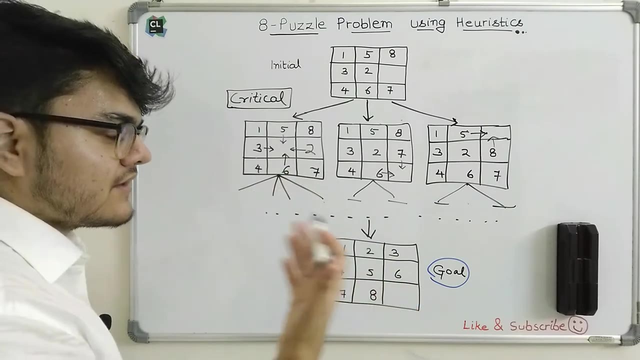 And you can see that this movement will cause the configuration to become the previous state. You can see, this is the same as this one, Right? So this type of moment we are not going to allow. Why? Because there will be some unnecessary states and unnecessary branches which we are trying to avoid. 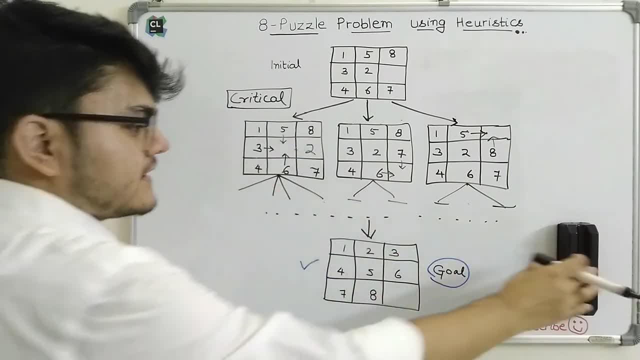 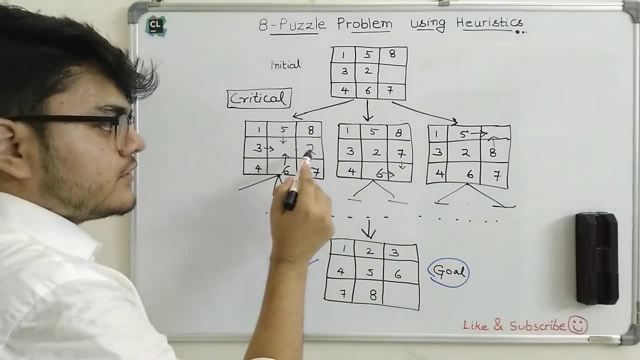